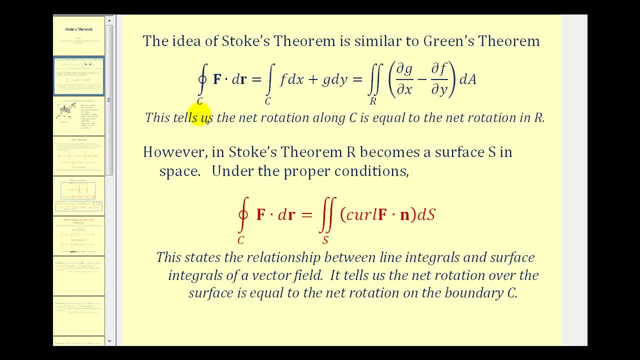 Remember. this tells us that the net rotation along the curve C is equal to the net rotation of the vector field in the region R, Where R is in the xy plane. However, in Stokes Theorem the region R becomes the surface S in 3D or in space. 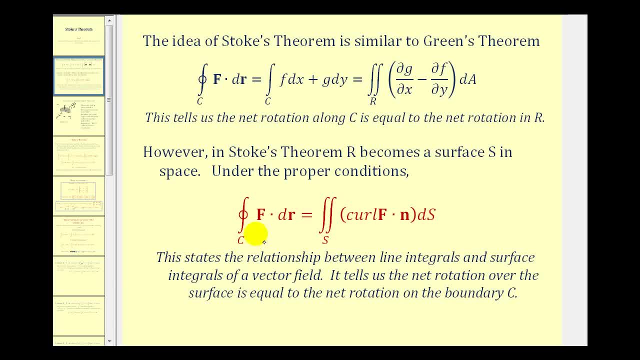 And under the proper conditions, we have this line integral here equal to the surface integral of the curl of F dotted with N. So Stokes Theorem states the relationship between line integrals and surface integrals of a vector field given specific conditions, And it tells us the net rotation over the surface. 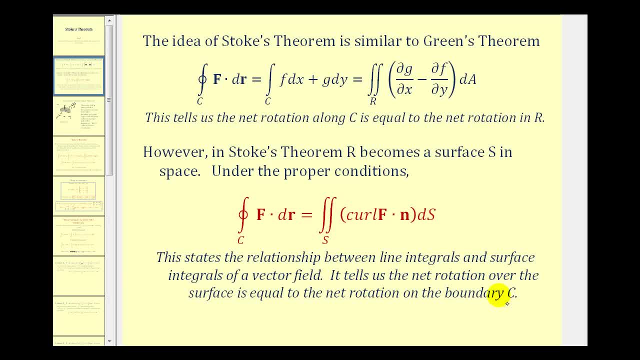 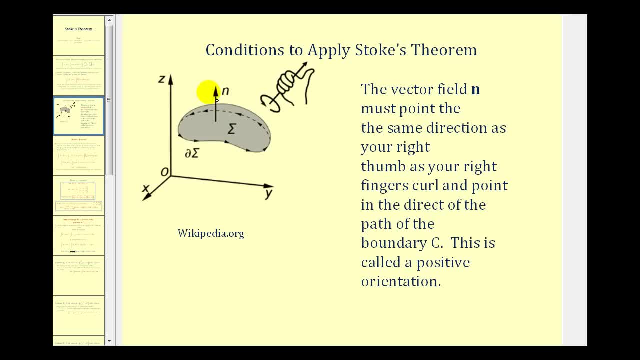 Is equal to the net rotation on the boundary C, given certain conditions. So let's now talk about the necessary conditions to apply Stokes Theorem. If we have our surface here in gray, The vector field N, the unit normal vectors, Must point in the same direction as your right thumb. 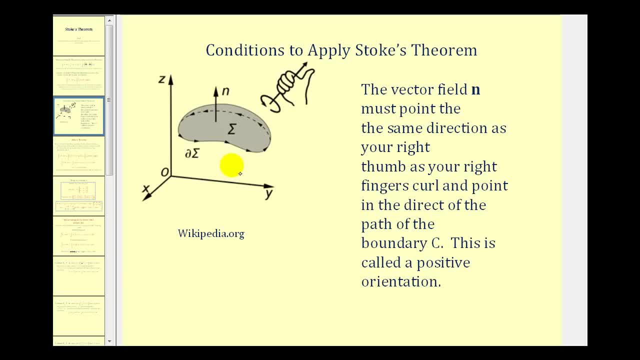 As your right fingers curl and point in the direction of the path of the boundary C. Looking at this diagram here, If our thumb is pointing upward In the same direction as the unit, normal vectors Notice- the fingers would point counter clockwise, Giving this the correct orientation. 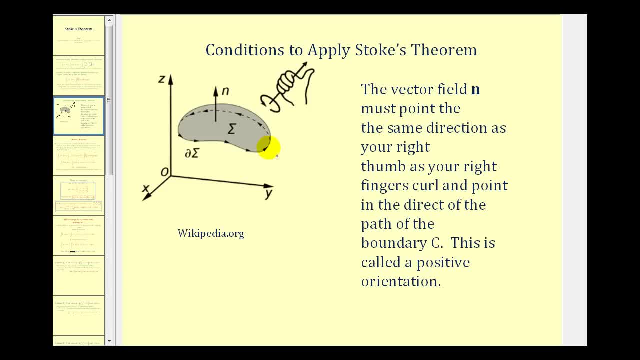 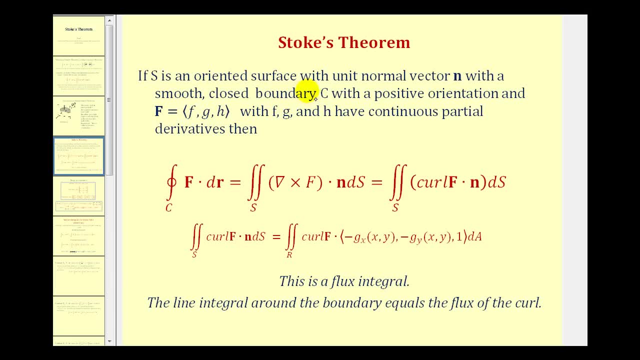 And this is called a positive orientation, Which is required by Stokes Theorem. Let's go ahead and formalize Stokes Theorem now. If S is an oriented surface with unit normal vectors N, And also having a smooth, closed boundary, C With a positive orientation. 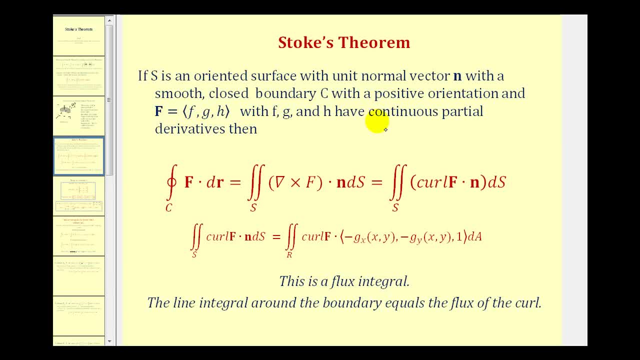 And the vector field F has components with Continuous partial derivatives. Then we have the line integral Of F dotted with DR Along C, Equal to the surface integral Of the curl of F Dotted with N DS. Remember the curl of F can be written like this: 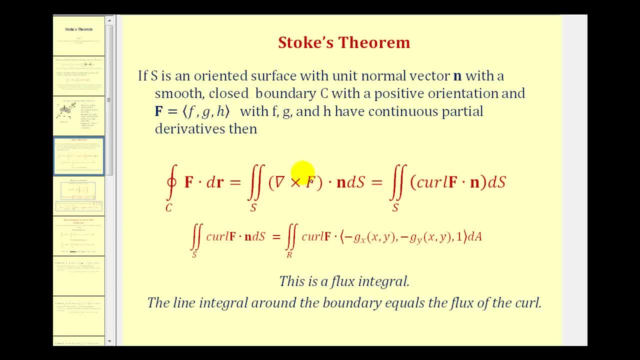 Or we can also think of it as Del cross with the vector field F, Because this form reminds us of how to determine the curl of F. Then remember from the video: on the surface integral of a vector field, N, differential S, Is equal to this vector field. here. 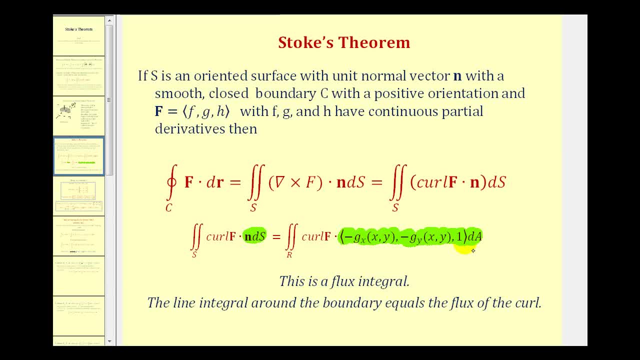 Times differential A, Given we have a positive orientation. Remember this really is just the gradient of big G, Where big G Is equal to Z minus G of X and Y, And because we have a vector field dotted with N, This is called a flux integral. 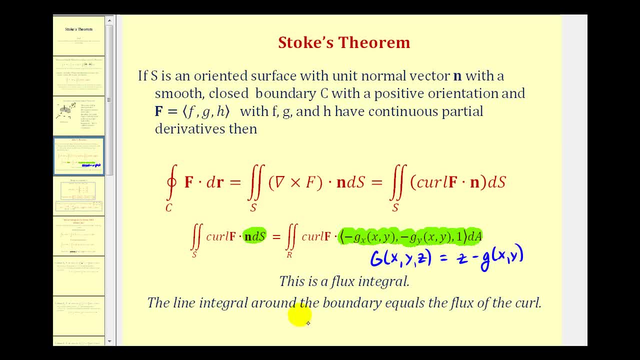 And so we can say that the line integral around the boundary C Equals the flux of the curl Over the surface S. Let's go and take a look at our first example, And, as mentioned before in this video, we're going to use Stokes theorem. 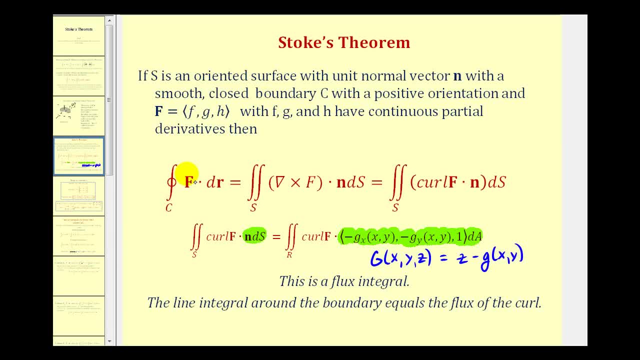 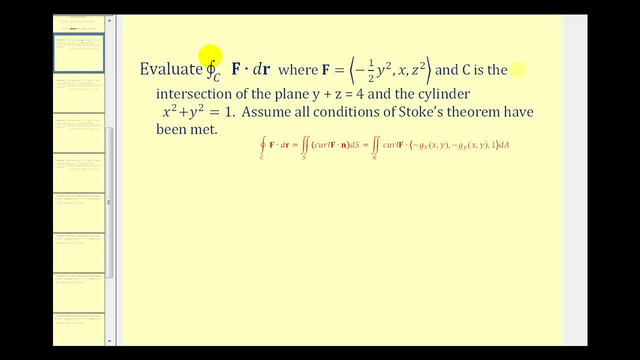 To evaluate a line integral. So we'll be given a line integral And we'll convert it to a surface integral. Let's go and take a look at our first example. In this example we want to evaluate the line integral of F dotted with DR. 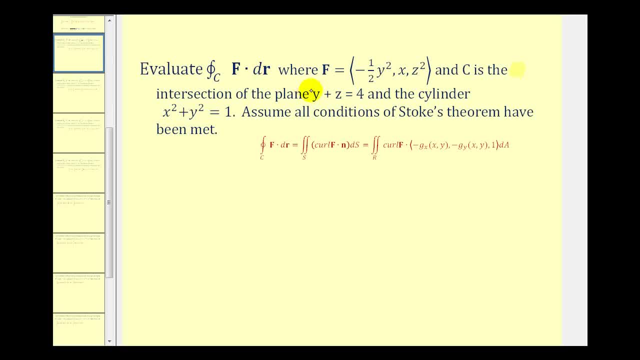 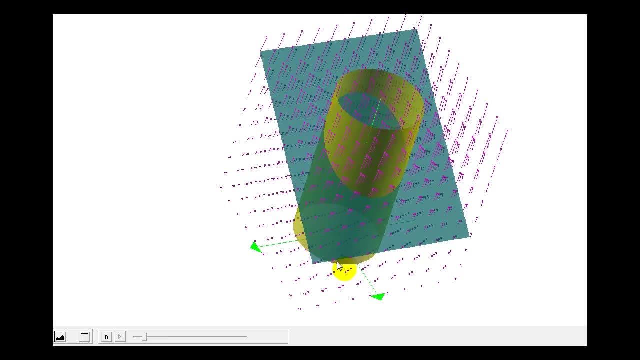 With the given vector field And C is the intersection Of the plane. Y plus C equals four And the cylinder, X squared plus Y squared equals one, And we'll assume all the conditions of Stokes theorem Have been met. Let's start by taking a look at the graph of this. 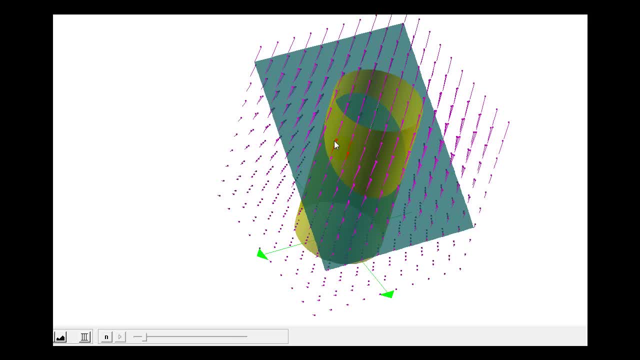 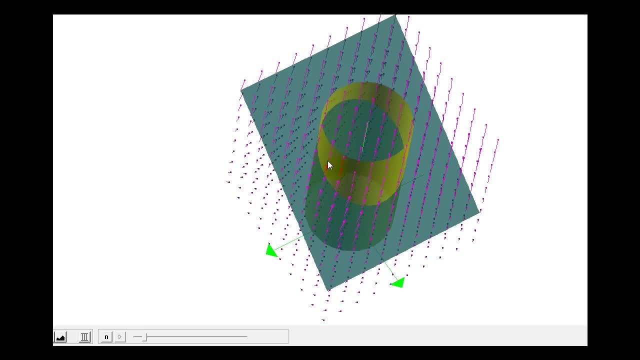 So our surface is the intersection of the yellow cylinder And the green plane. So we'll use Stokes theorem to evaluate the given line integral, Which will tell us the net rotation. This is by the vector field, Which is the intersection of the cylinder and the plane. 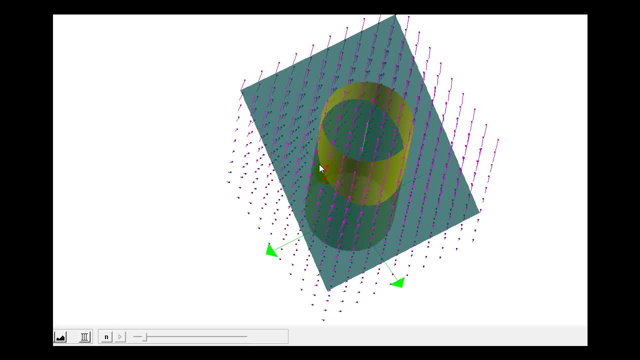 With a counterclockwise orientation, Which is also equal to the Net rotation of the vector field over the surface, And if it's positive, that means the net rotation would be counterclockwise And if it's negative, The net rotation would be clockwise. 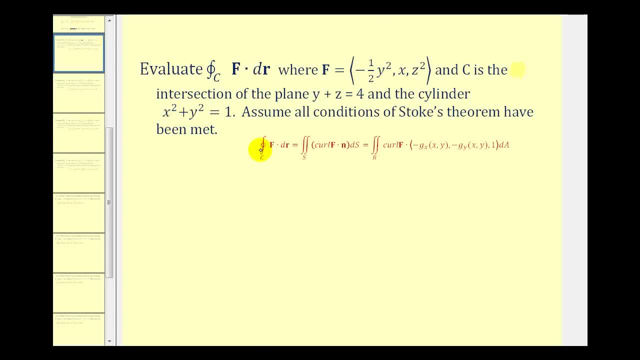 Based upon the given orientation. So to evaluate this line integral We'll apply Stokes theorem And evaluate this surface integral instead. So we'll start by determining the curl of the vector field F. So we can use a three by three determinant Where the first row will be IJK. 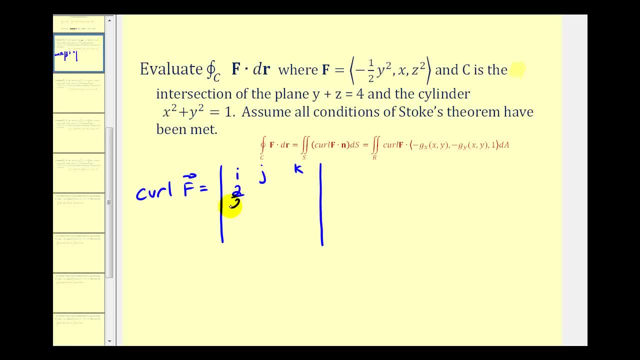 The second row will be the partial derivative operators. The third row will be the components of our vector field. We'll go ahead and use the cofactor expansion method this time. So for our first two by two determinant, We'll eliminate row one and column one. 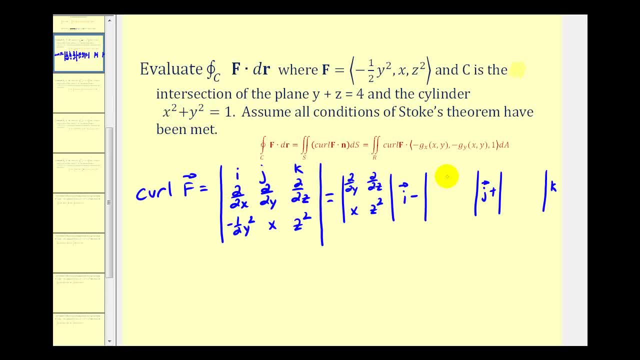 For our second determinant, We'll eliminate row one and column two, And then for our third determinant, We'll eliminate row one and column three. So here we'll have the partial derivative of Z square with respect to Y, That'll be zero. 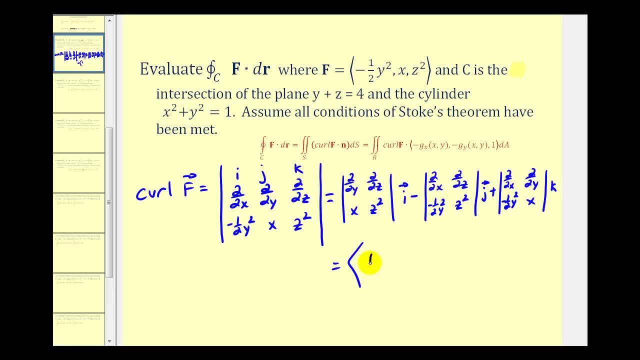 Minus the partial derivative of X with respect to Z, That's also going to be zero. Here we'll have the partial derivative of Z square with respect to X. That's zero, Minus the partial derivative of negative one half Y square with respect to Z. 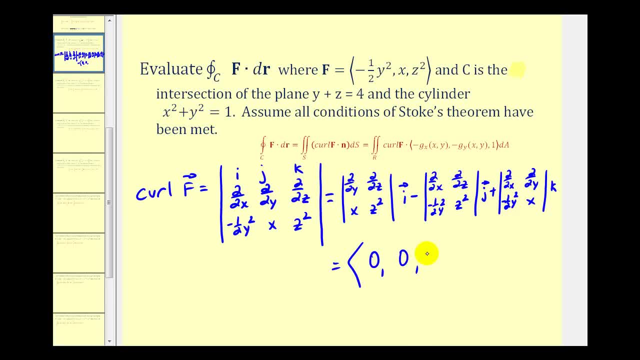 That's also zero. And then, for our Z component, We'll have the partial derivative of X with respect to X- That's going to be one- Minus the partial derivative of negative one half Y square with respect to Y- Well, that's going to be negative Y. 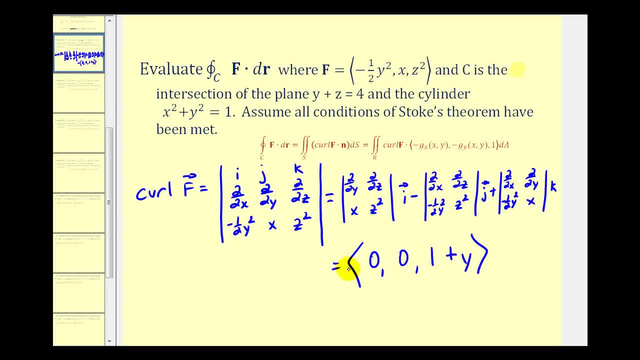 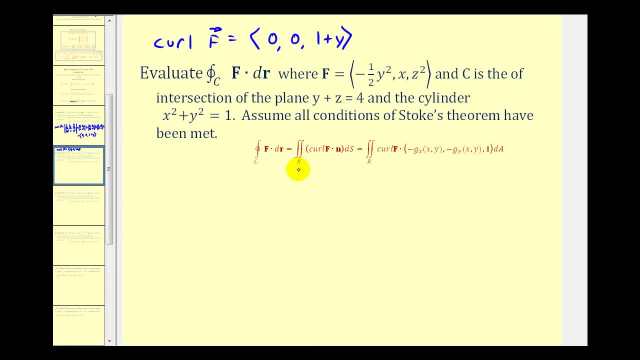 So minus the negative Y will be plus Y. So here's the curl of F. Now to evaluate this surface integral, We're going to convert it to a double integral over the region R, And so we'll have the curl of F dotted with. 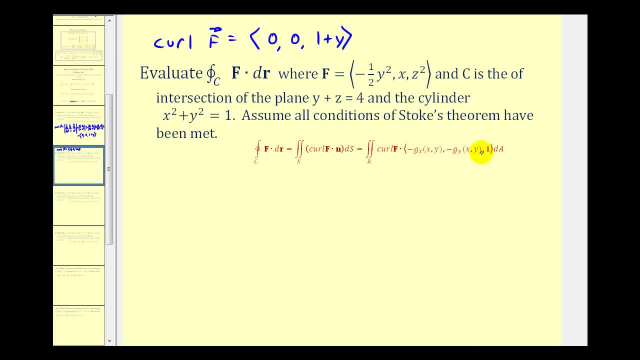 This is the shortcut for the gradient of big G, Where big G is equal to Z minus G of XY. Or we can say that Z is equal to G of XY, Which in this case, given by the plane, is going to be equal to four minus Y. 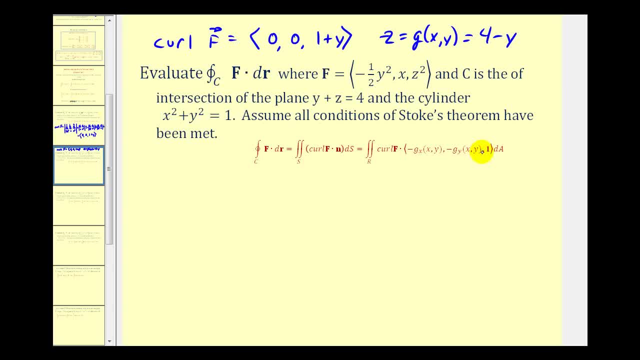 So we'll use this for the shortcut of our second vector field. So we're going to have the curl of F Dotted with the opposite of the partial derivative of G with respect to X. Well, that's going to be zero, The opposite of the partial derivative of G with respect to Y. 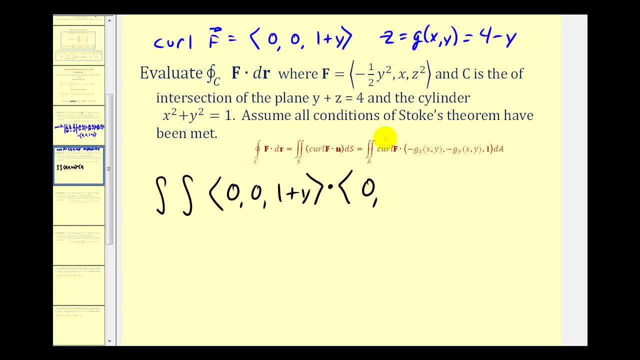 Well, the partial derivative would be negative one, And then the opposite of that would be positive one, And then the Z component is always equal to one. Given our orientation, Let's go determine our dot product. So we have zero plus zero plus one plus Y times one. 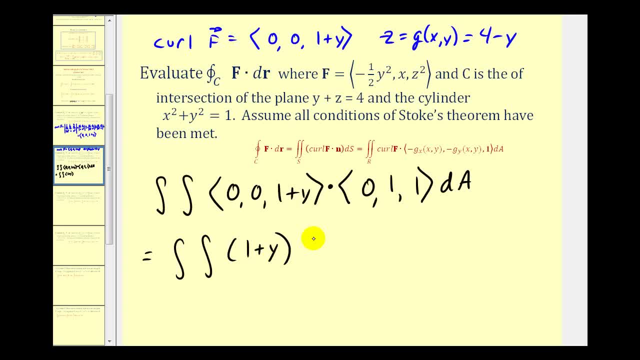 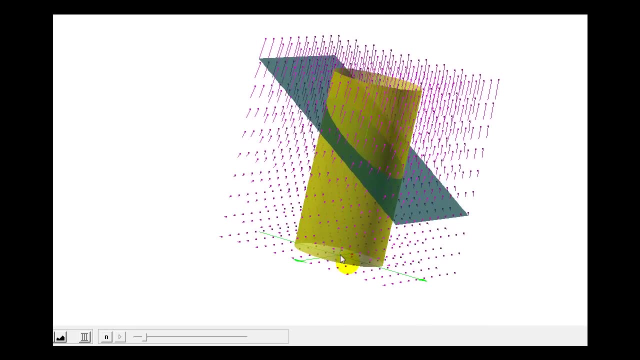 That's going to be one plus Y. Now for differential A. let's go ahead and sketch our XY trace. Let's go back and take a look at our graph real quick. The XY trace of our surface, As you can see here, would just be this circle here. 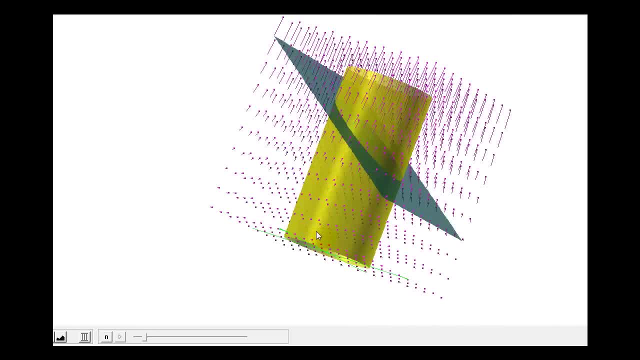 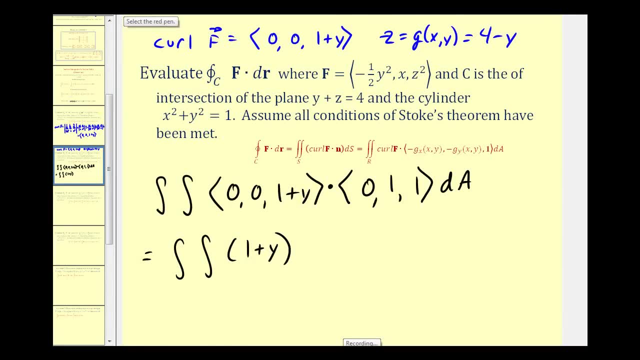 Determined by the cylinder. Let's go ahead and sketch that. Since our XY trace is a circle, We're probably going to want to use polar coordinates. Let's go ahead and sketch it. So, for differential A, let's go ahead and rewrite this as: 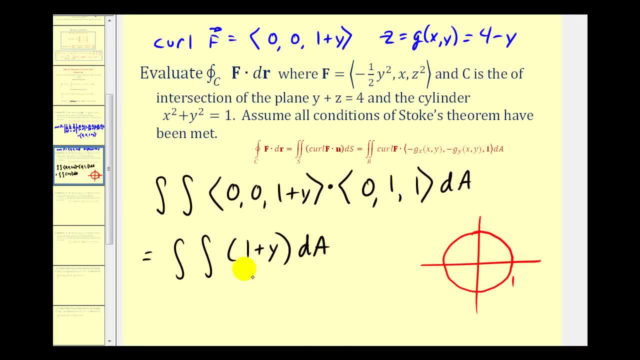 R D R D theta. And then we use our sketch here to determine our limits of integration. So we'll have one plus Y is equal to R sine theta, And remember that differential A In polar form would be R D R D theta. 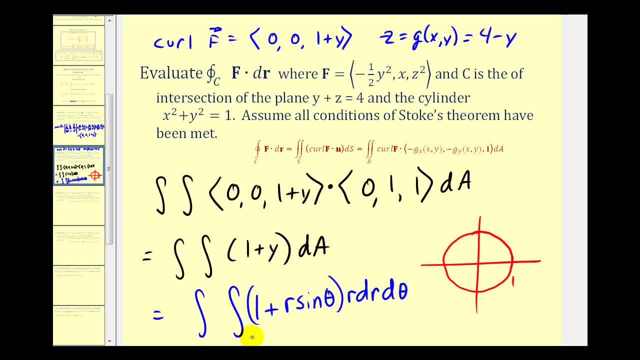 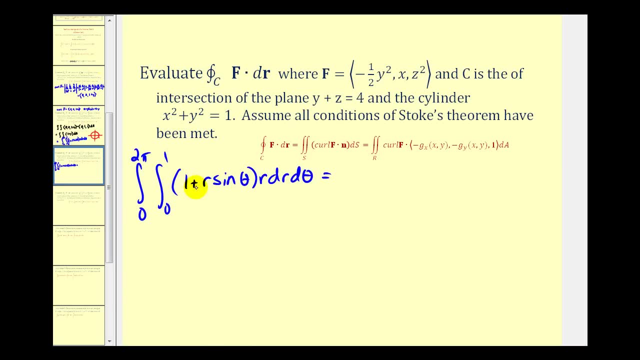 So the limits of integration for R would be from zero to one And theta would be from zero All the way around to two pi. Let's go and evaluate this on the next page. Let's go and distribute here. So we have R plus R squared sine theta. 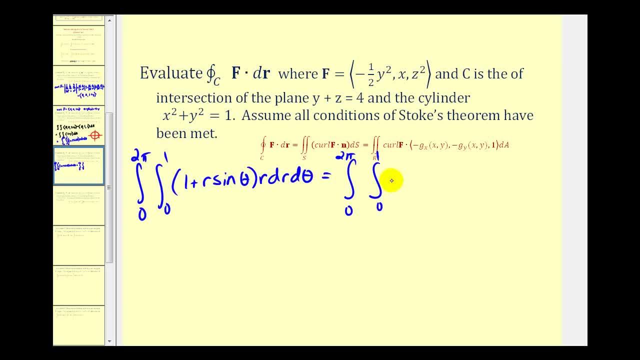 So we're going to have R squared over two Plus R cubed over three, sine theta. Subbing in R equals one, we'll have one half Plus one third sine theta. And then when R is zero, we'd have zero, So we'll have one half theta.